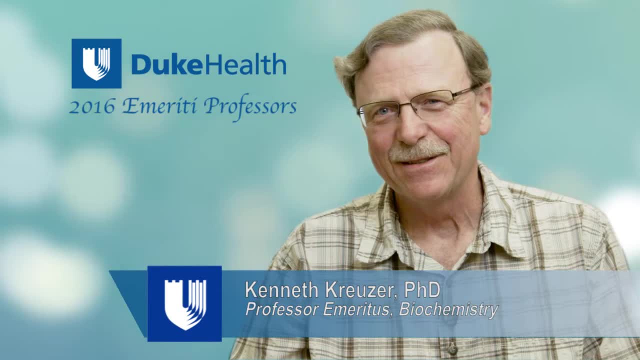 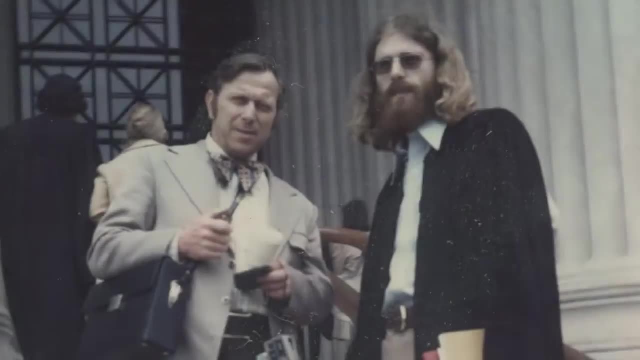 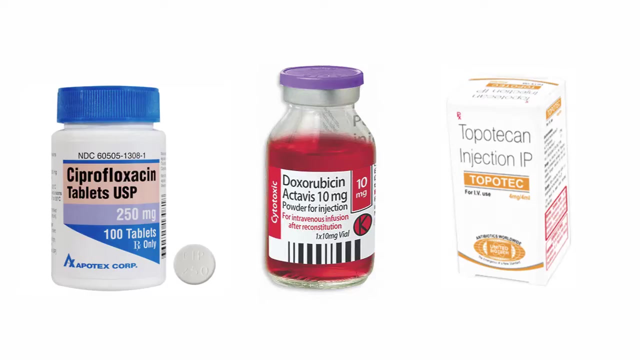 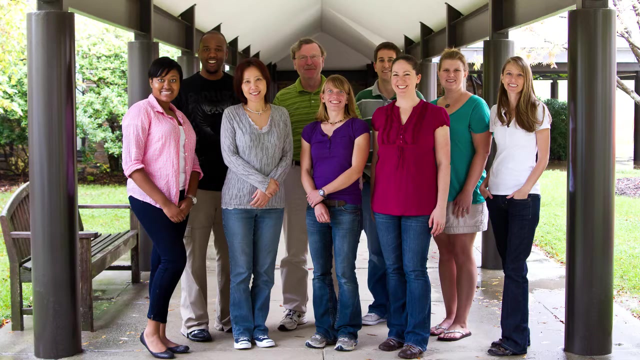 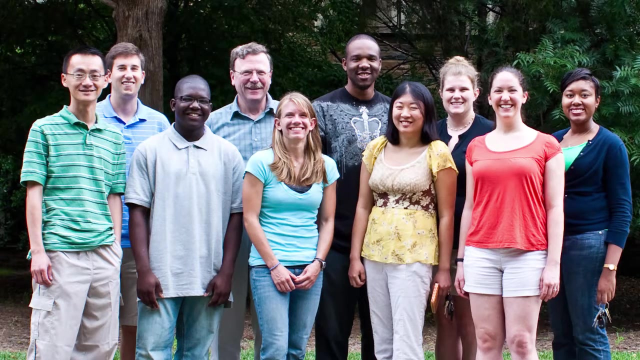 As a young researcher, Ken Kruiser was the first to show that certain drugs convert an important cellular enzyme into a toxic product that prevents DNA replication and kills cells. This discovery and subsequent research by his and other labs have refined the mechanism and use of several important classes of anti-cancer and anti-bacterial drugs. 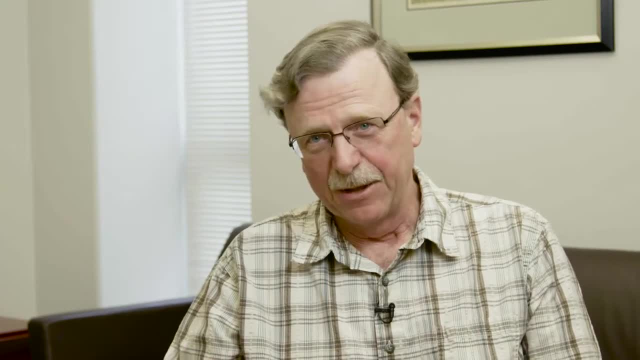 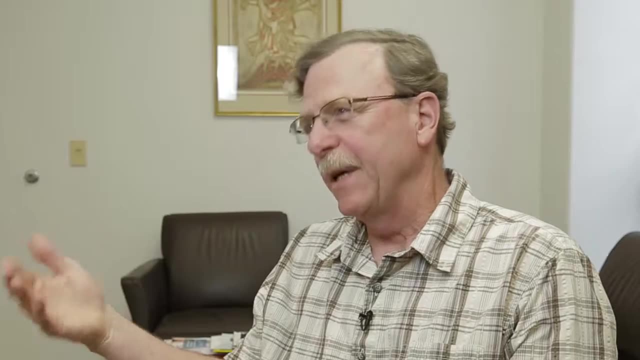 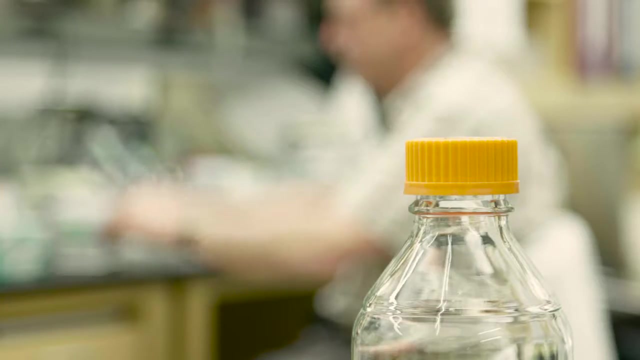 And so over the years we've been involved in multiple studies and other labs have as well, trying to understand exactly how that protein DNA complex really messes cells up and how they try to respond to it, And that's work that's still ongoing in a number of labs. 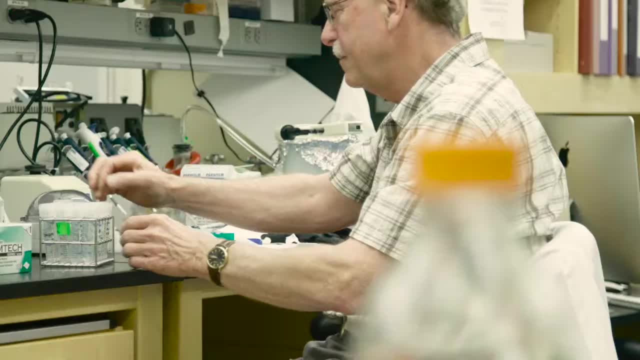 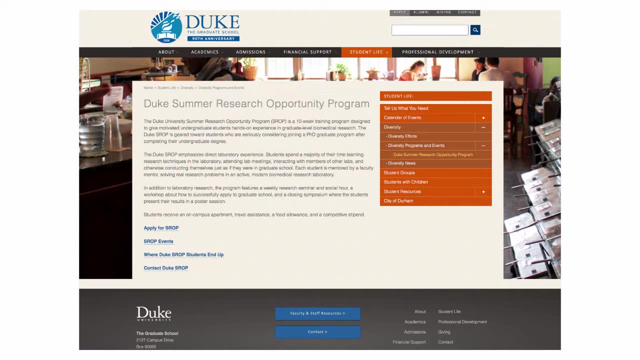 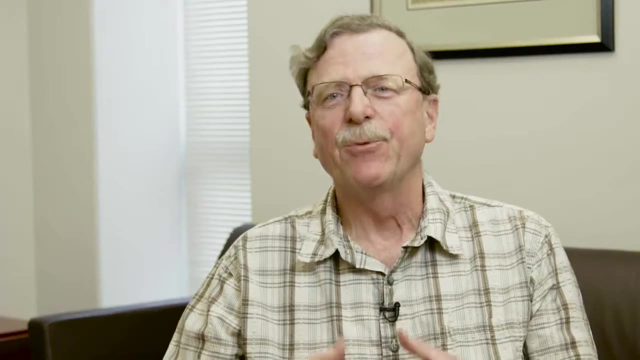 Away from the bench. Kruiser has been a passionate advocate to attract more underrepresented minorities to the medical sciences. He pioneered Duke's Summer Research Opportunity Program, which is now more than 20 years old, And we've trained well over 200 students in the program. We give them research opportunities. 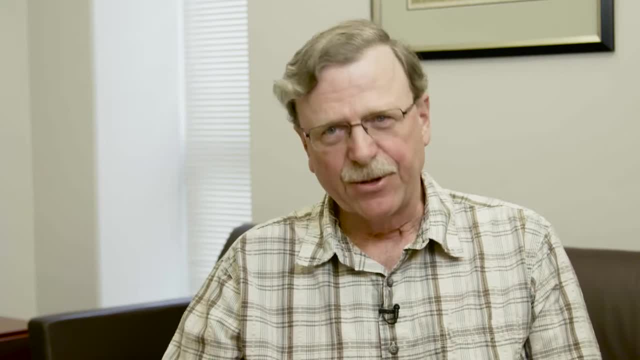 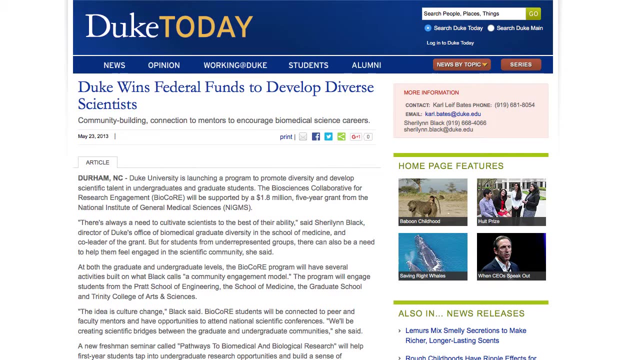 for 10 weeks in the summer and also a lot of seminars about career development and things like that. Along with Sherrilyn Black and Julie Reynolds Kruiser, co-created a program called BioCore, which is partially funded by the NIH to support undergraduate and graduate research for underrepresented 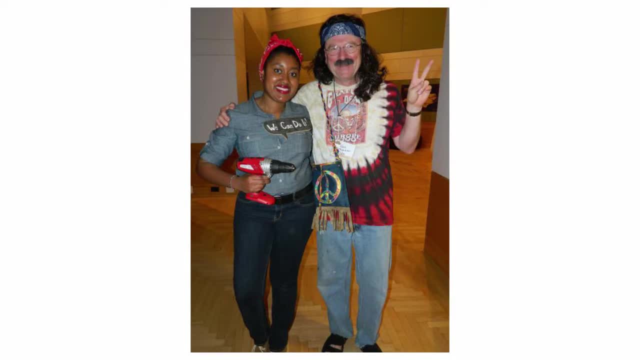 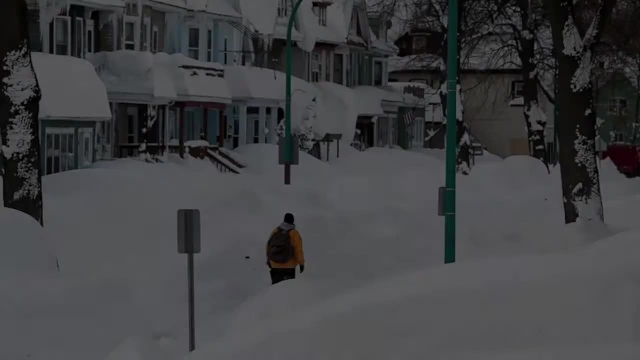 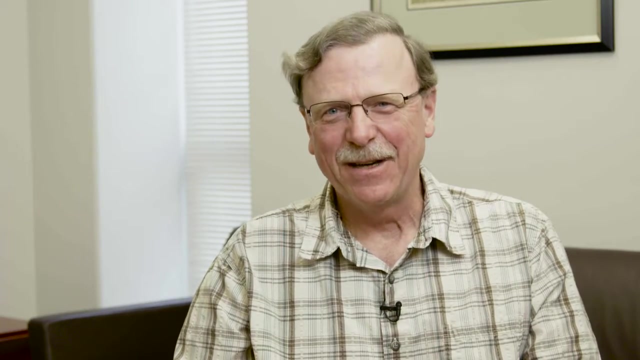 minorities And it's just been incredibly rewarding to see, you know, hundreds of kids, really, you know, getting to experience science. Kruiser was raised in Buffalo, New York. before heading off to college It was pretty miserable up there, after about five months of snow and cold. 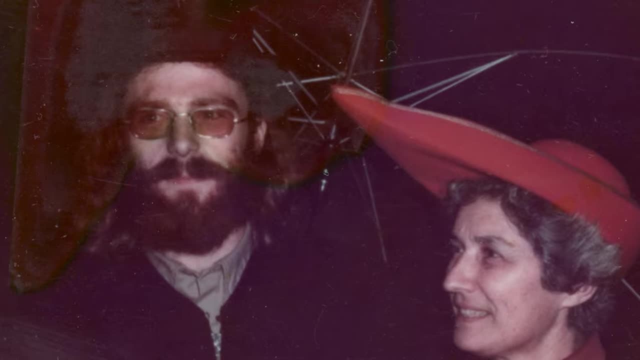 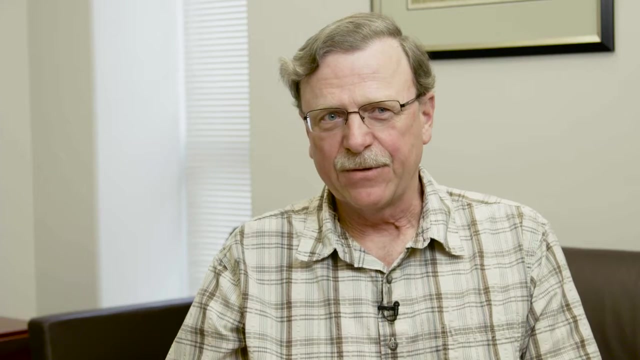 He has always been interested in science and it was as an undergrad at MIT where he was bitten by the research bug. And what was then? the research bug? I took a course from a guy named Salvador Luria- who got the Nobel Prize, actually- and 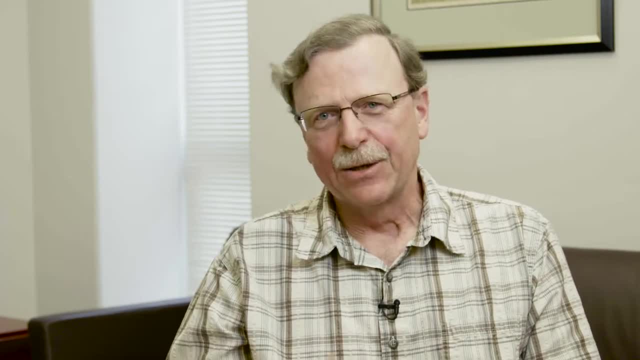 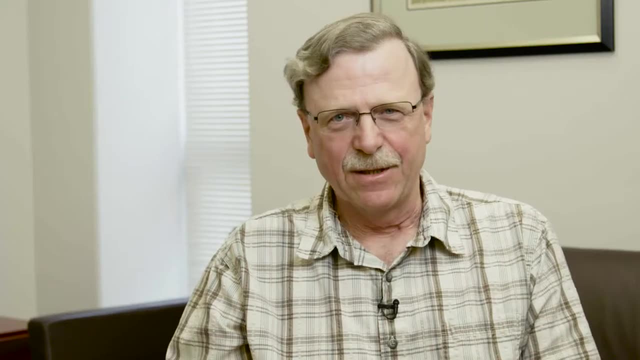 he was just absolutely inspirational, showing how you could learn about what's going on with the DNA molecule by looking at the color of colonies on petri plates, And so in that course I kind of learned that it was actually possible to figure out things about how life works at the molecular level.